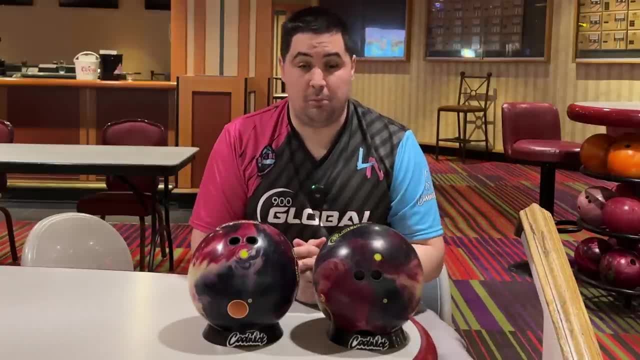 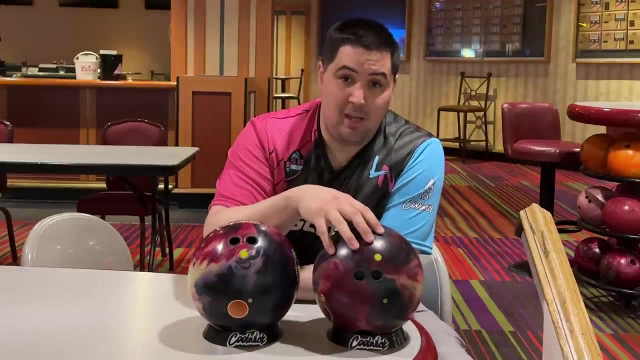 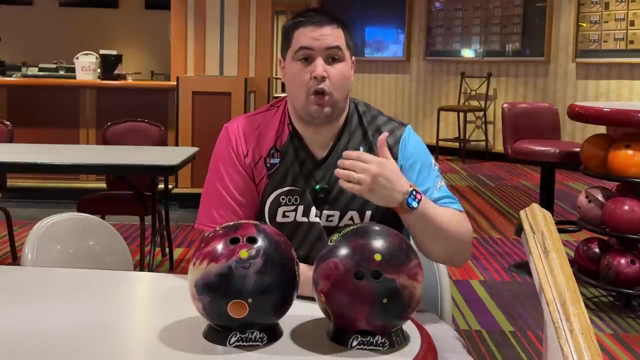 the fingers. then it is going to be a pin up bowling ball. Now what does that actually do to ball performance? So a bowling ball that's drilled, pin up is actually going to increase the differential and decrease the RG. The higher the differential, the more hook potential. 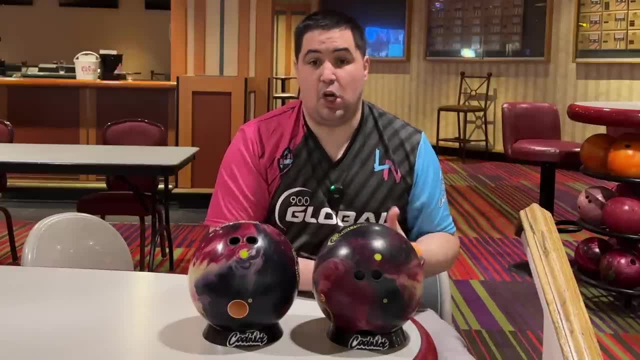 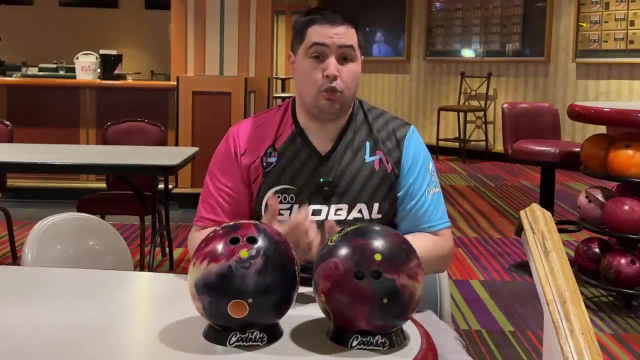 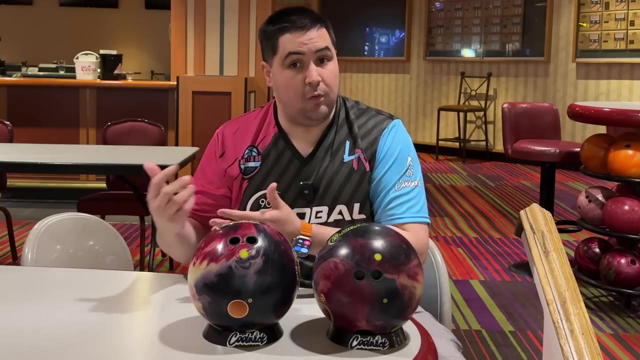 the bowling ball has, then the lower the RG, the earlier the ball is going to want to start up and and and how much and how quick it's going to respond to that friction. So if you drill your bowling ball pin up, it's going to hook more or have a higher hook potential, and it's going to 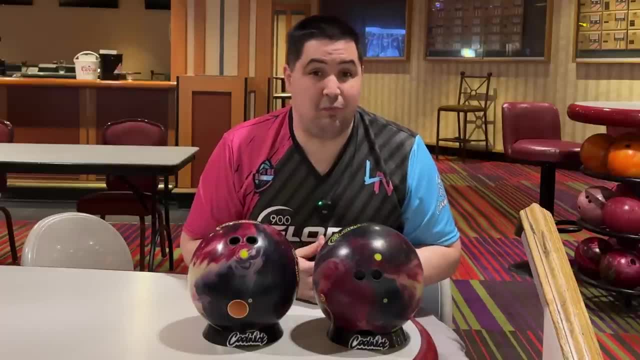 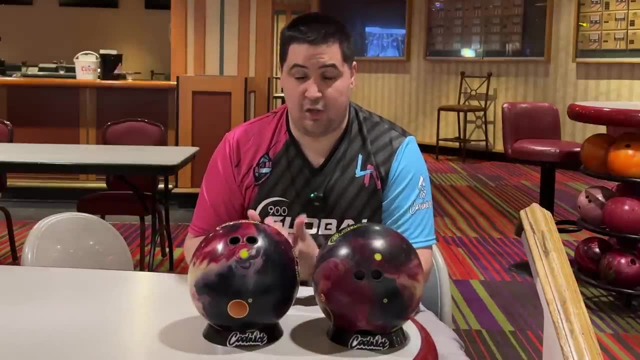 want to get started earlier and respond quicker to the friction. And then when you drill your pin up, you're going to have a higher hook potential and it's going to be just the opposite: It's going to decrease the differential and then it's going to increase the RG. 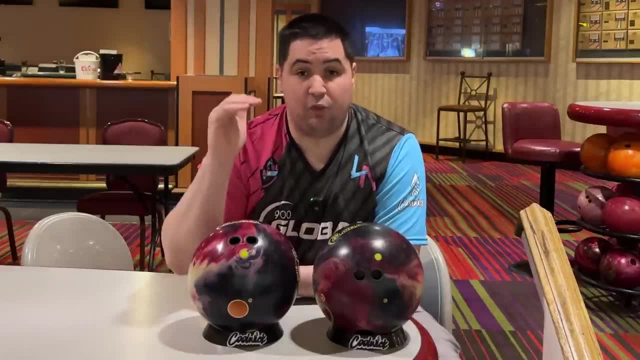 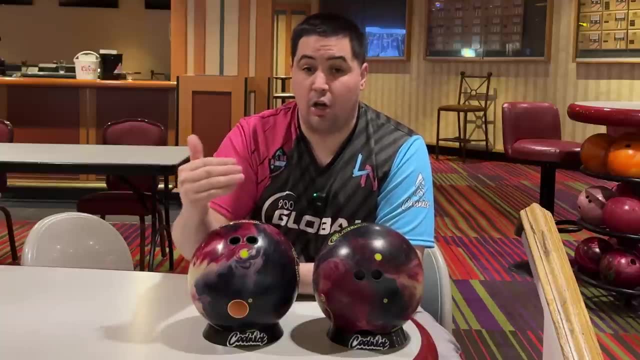 So when you drill a pin down, the hook potential of the bowling ball is going to go down and the RG is going to go up, meaning the ball is going to want to be a little bit longer before it makes its motion and it's also going to make it a little bit smoother. So pin up is going to make the ball. 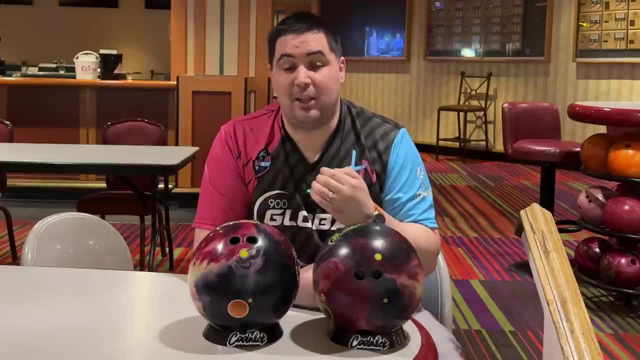 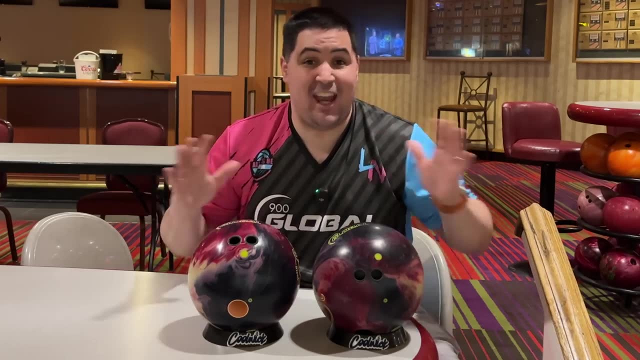 hook more and earlier. So when you drill a pin down it's going to be just the opposite. It's going to make the ball go a little bit longer and be a little bit smoother down lane. Now, all of that can change with surface anyway. So if you drill your ball pin up and it's hooking too early, you 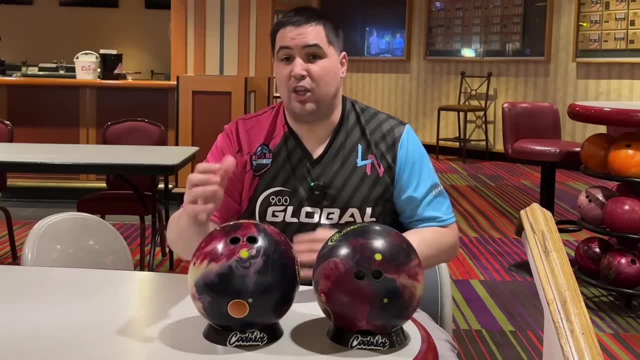 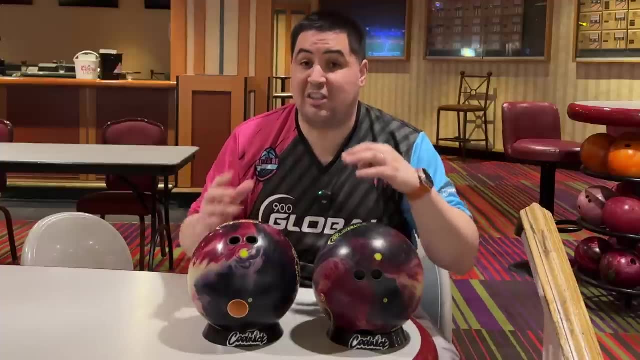 can always polish it up. Same thing with pin down. If it's a little bit too long and you need it to be a little bit earlier, add more surface. So the surface is always going to be the biggest thing. but today we're going to talk about just the layouts. So in front of you here you have two. 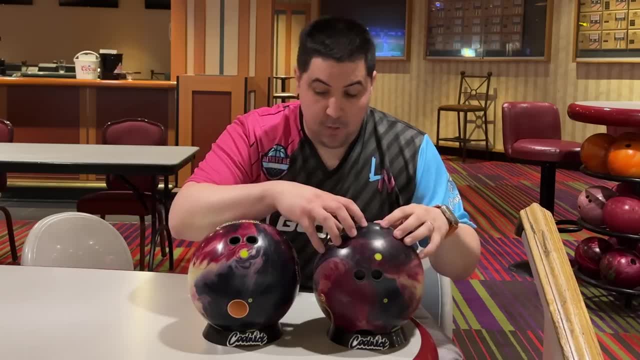 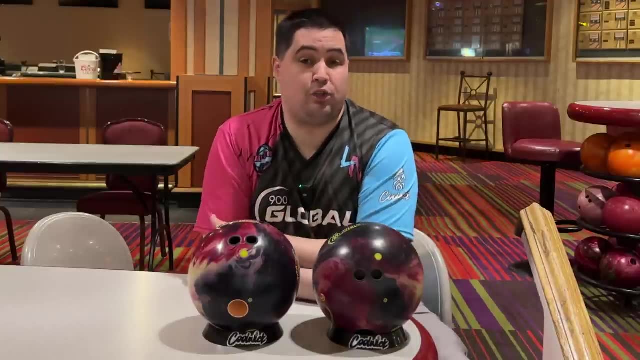 900 Global Eternity Pis: One drilled pin up, one drilled pin down. So if you're looking for a ball hook, you're going to be here at Samstown on lane 42 on a fresh, typical house shot. The question that I have for you guys is: do you prefer pin up drillings? Do you prefer pin down drillings? 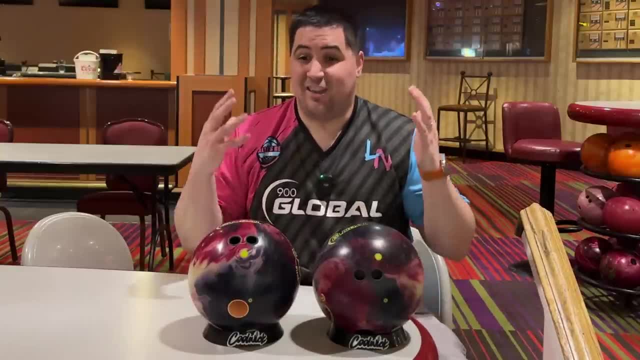 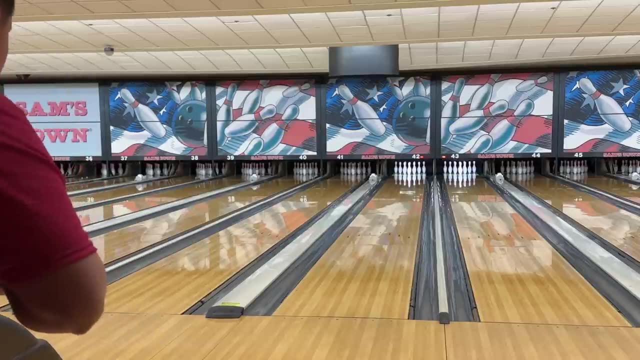 Why, or why not? Or are you learning about this for the first time? Because that's kind of what I want. I want to educate as many people as possible. We'll see you here on the lanes. All right, first shot of the video. we're going to start in the pin up: Eternity Pine Before I get in the pin down. 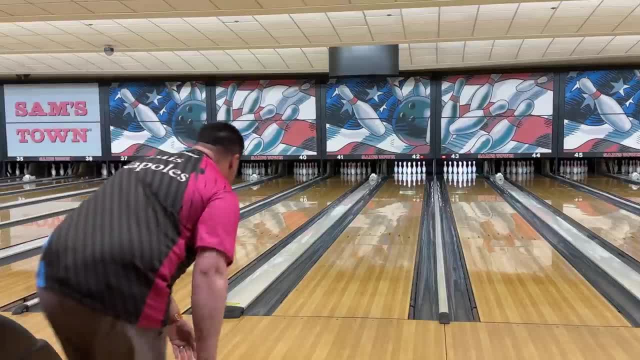 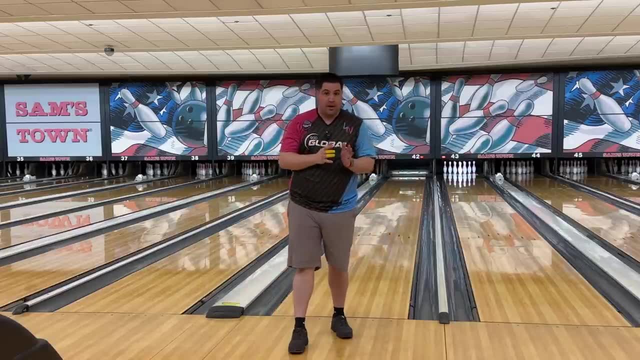 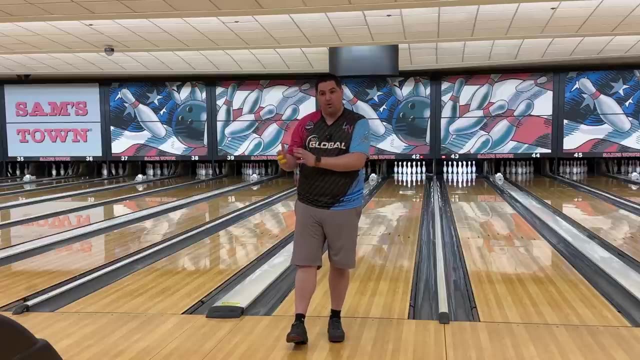 I'll make sure to let you guys know. Yeah, so the biggest thing to pay attention when looking at that shot is how much earlier it wanted to pick up and that motion down lane. When we get to the pin down one, you guys are going to see. 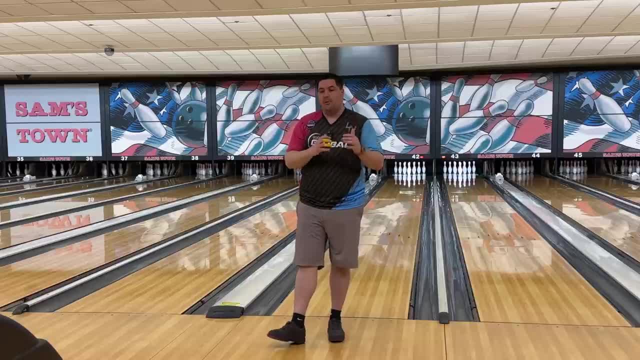 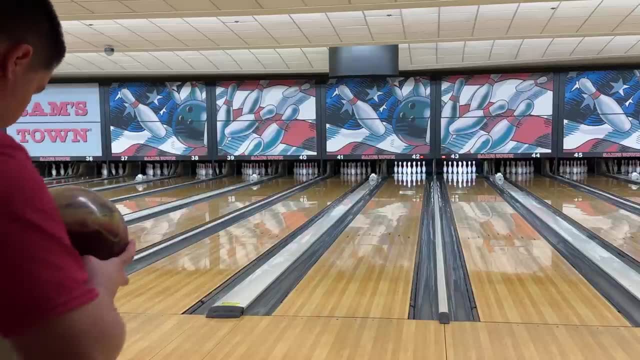 that it's going to be very different. So right now I'm going to throw a couple more shots of the pin up one, and then we'll get into the pin down one. All right, then, the best advice I can give you guys is consult with your local pro shop operator to determine if pin up or pin down will be better. 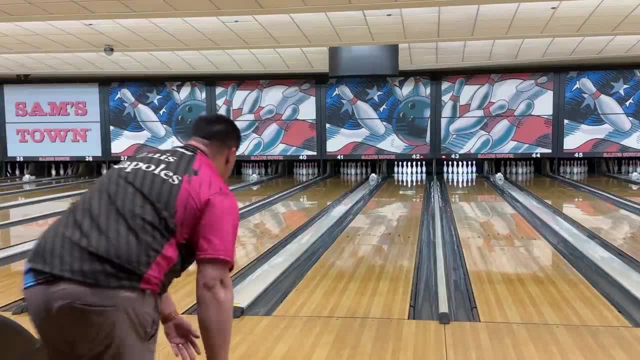 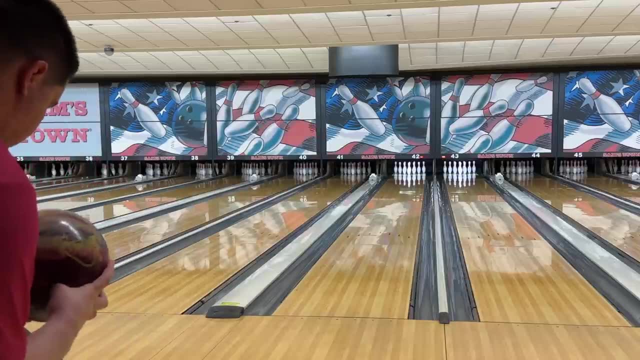 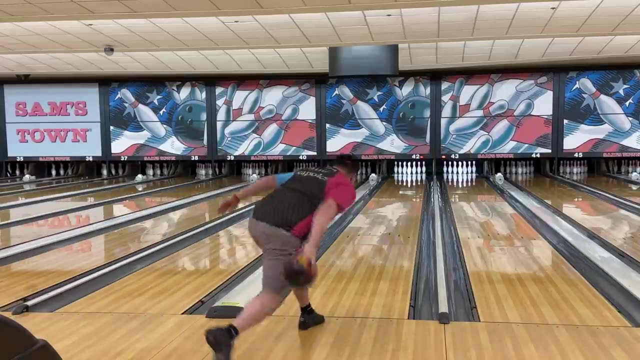 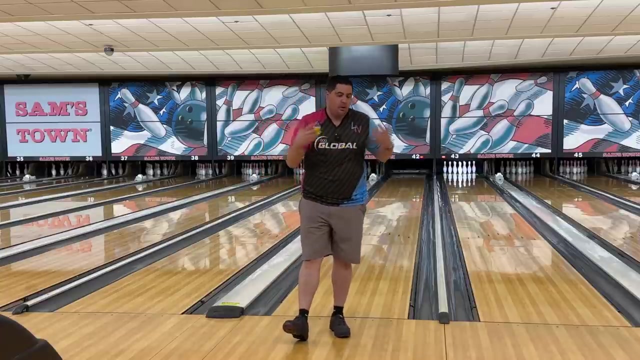 for your game. All right, one more here with the pin up one, and then I'll get into that pin down one. Got that a little right and I mean it is an asymmetrical solid, so it's not going to shape like a pearl, but for a solid you can see that it wants to get there and make a little bit more. 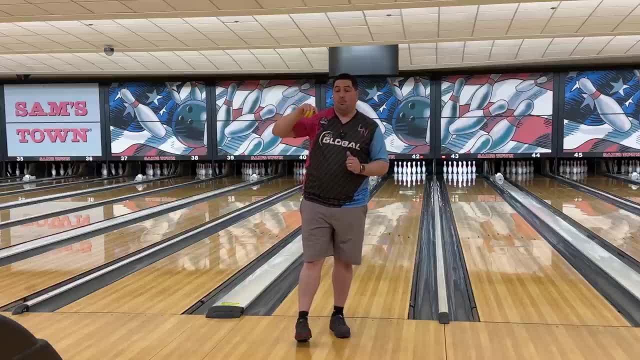 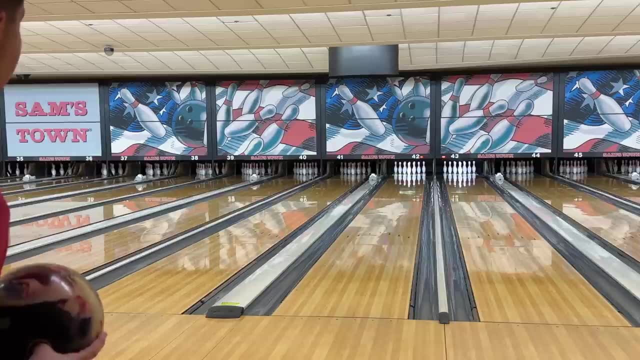 motion. The next shot you guys are going to see is the pin up one. So I'm going to get into that pin up one. I'm going to get into the pin down eternity pie, All right. so this is going to be the very first shot here with the pin down one. We're going to go right to that same spot to start. 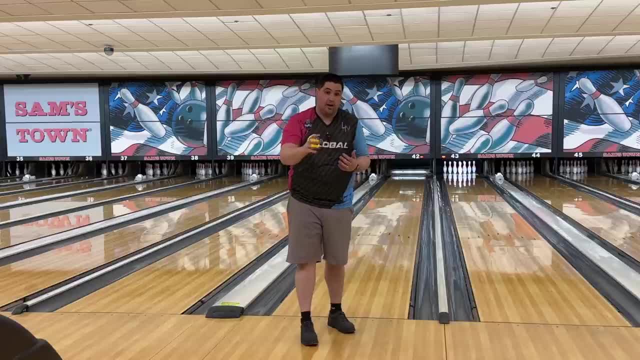 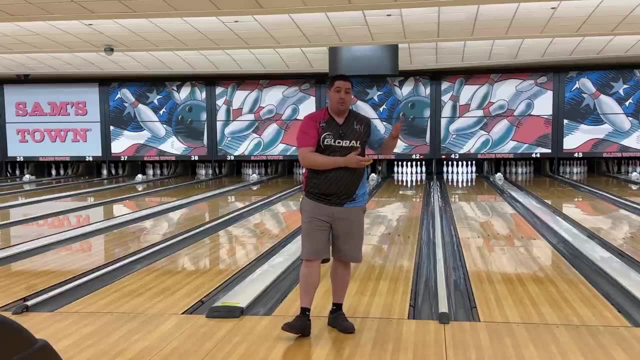 Yeah, I mean, I hope you guys can see just how much longer and smoother that was when compared to the pin up one. and right here, to my left or to your right, I'll show you guys what the pin up flare lines look like. and over here the pin up one is going to be the pin down one, So I'm going to get. 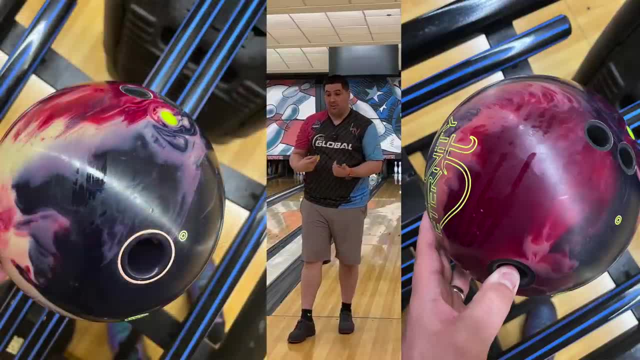 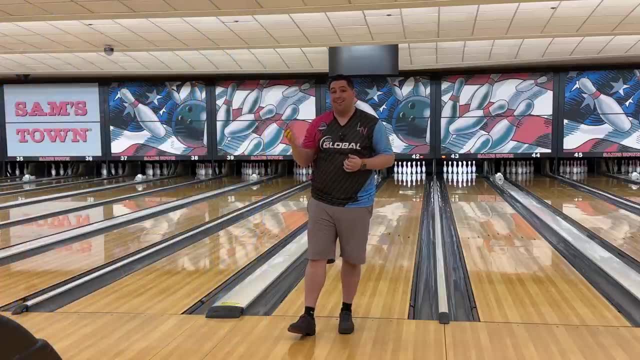 to my right, your left, I'll show you what the pin down flare lines look like. So night and day, as you guys can see, with the exact same ball, same surface, just really one pin up versus one pin down. Let's make a couple more shots there. All right, so that was a pretty good shot, so we're going to stay in. 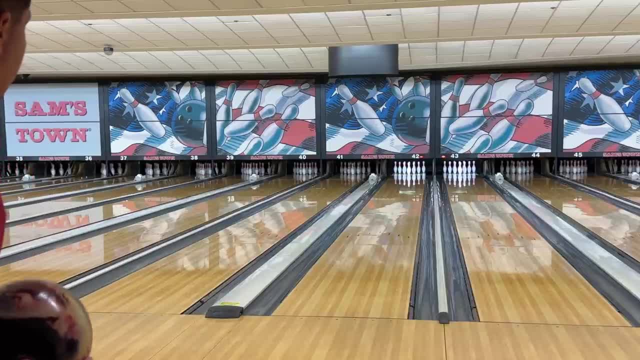 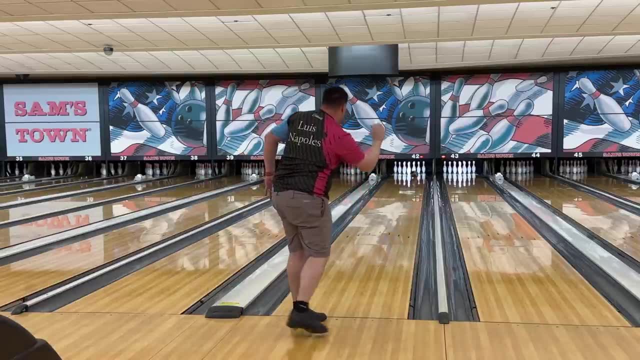 the pin down one same spot, repeat another good shot. So I actually got that one in a little bit and it held and I don't think that's going to happen again. So I'm going to go right to that one and I'll show you guys what the pin up one is going to look like. So I'm going to go right to that. 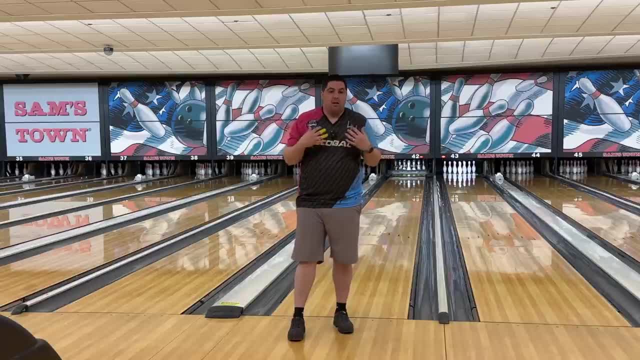 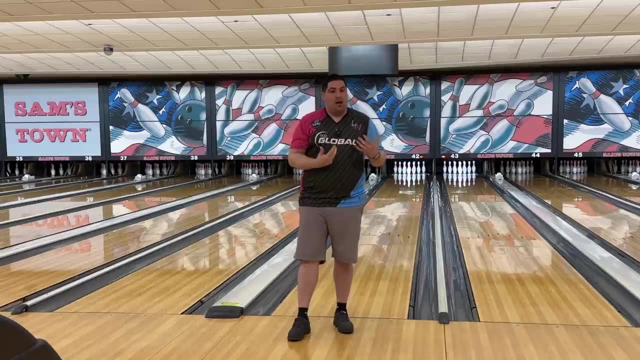 pin up one. I think that the pin up one would have held from that spot. So what I look for to determine whether I'm going to throw, like the pin up eternity pie or the pin down one, is if I'm bowling on a house shot, kind of like here at Samstown, where there's a lot of friction to the right, I think. 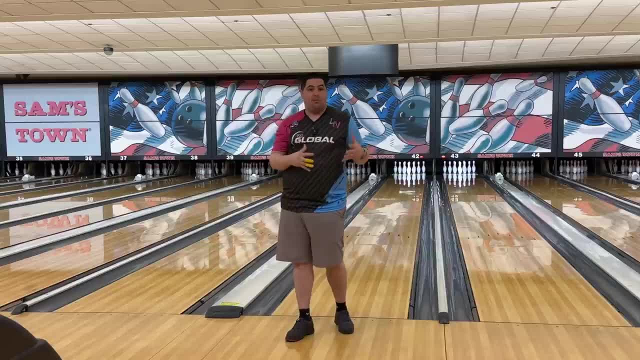 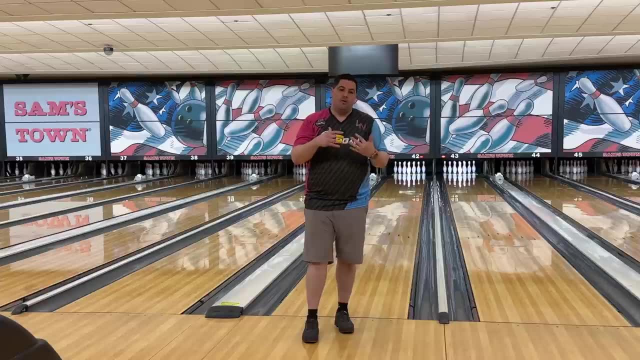 I'm going to end up liking that pin down one a little bit more. It'll allow me to play a little bit straighter, more mis room, whereas that pin up one is going to be a ball that I'm going to use more when there's more volume, when I have to get in and play in that soup in the middle. 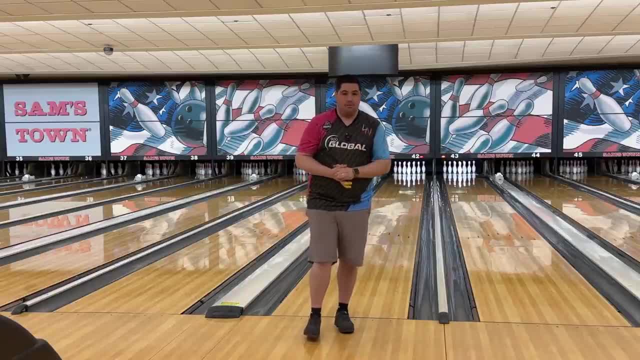 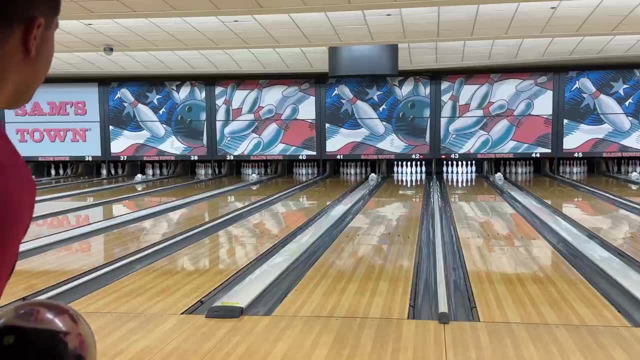 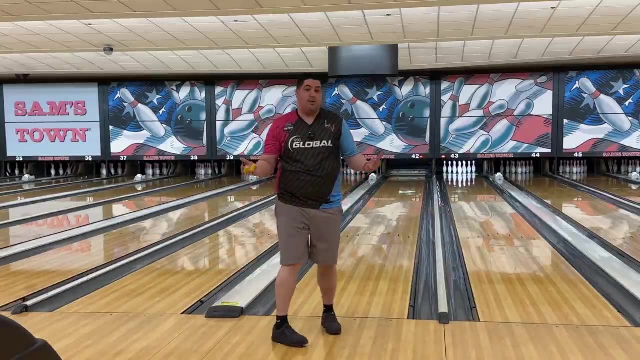 That's when the pin up one's going to look really good. So we'll do one more with the pin down one. All right, let's really focus. we get this pin down one going to the right, like we did with the pin up one, Like there. Now you can see, even though I mean I'm six for six to start it's way smoother. 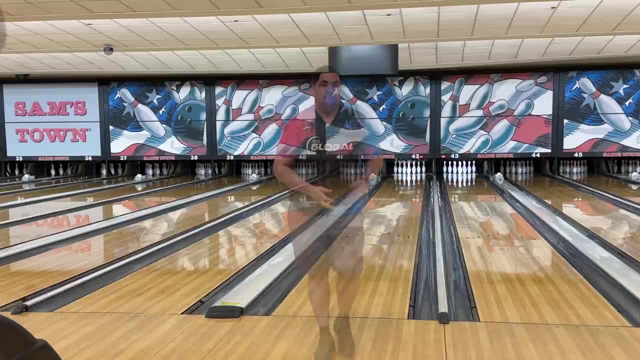 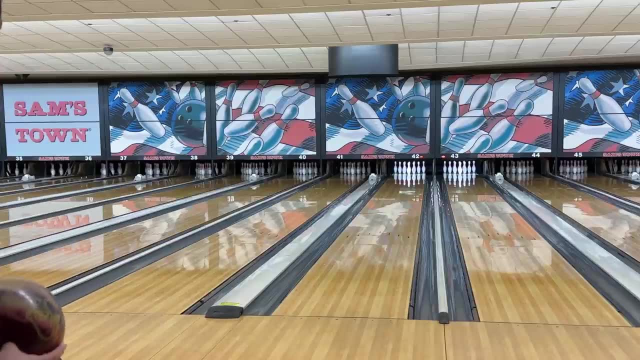 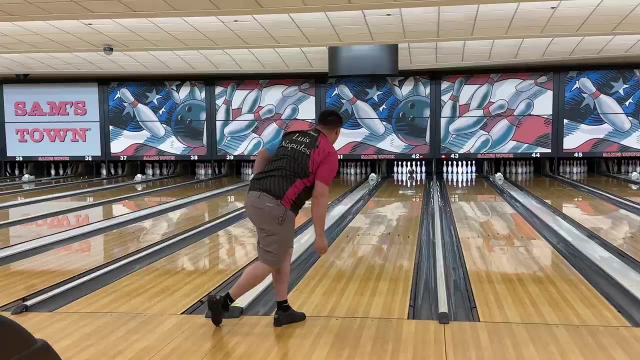 down lane more round. So let's get back into the pin up one now. All right, so this is going to be the pin up one, and we're going to move a zone left, a full arrow left, create a little bit more shape and see how they compare now. Yeah, I mean this. this bowling ball is disgusting, So let's get. 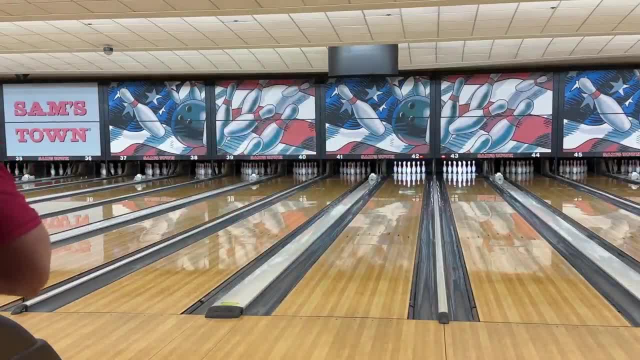 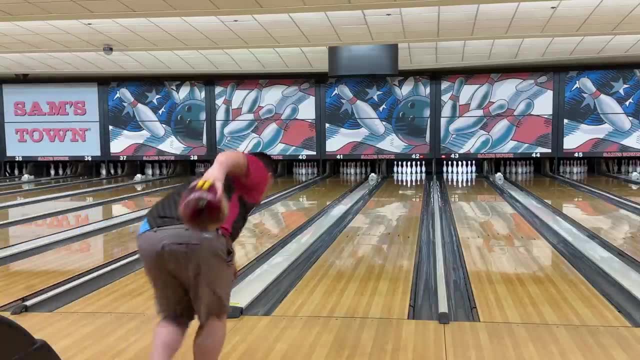 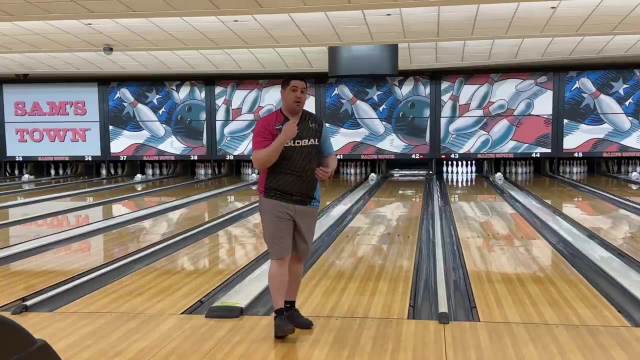 into the pin down one from there. All right, so this is going to be the pin down one from the same spot. for the sake of comparison, Let's see how this looks here, See if it gets there. Yeah, I mean, it's still struck, but you can see it really, really. 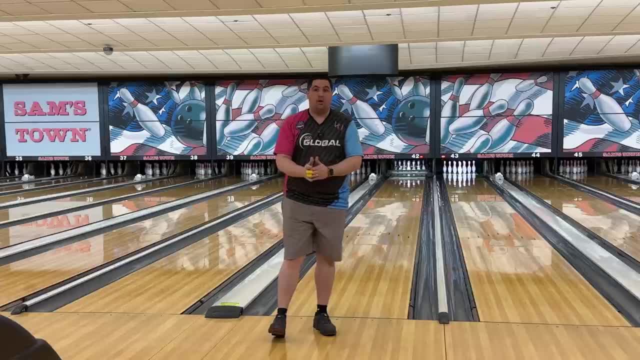 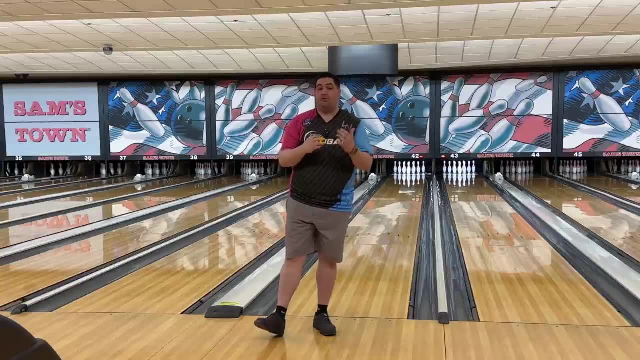 struggled to get there. So I'm going to stay in the pin down one and move straighter. keep my angles a little bit more in front of me so you can see more or less where I would like to play with this pin down one. So if I was bowling for score, I would be at this spot here with the pin. 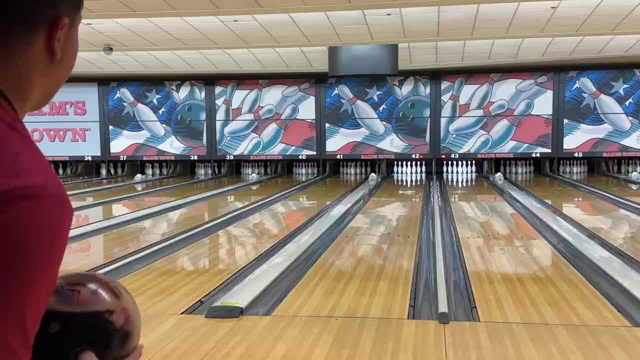 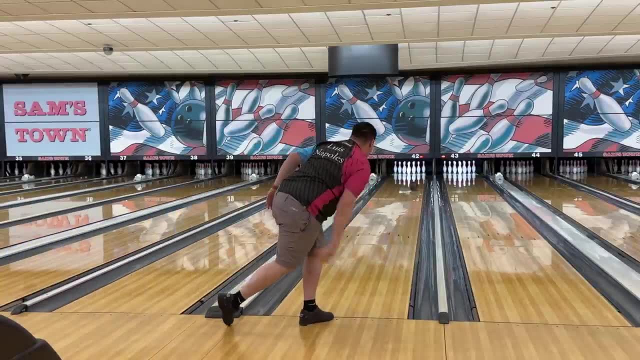 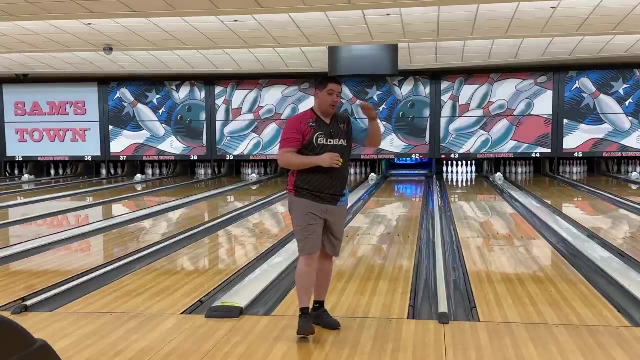 down one. I'm about 23 with my feet to start trying to hit like eight, nine, ten down lane. Yeah, like picture perfect. that's exactly where I was going to be. That would be with the pin down one. You can kind of see the differences there between the up one.